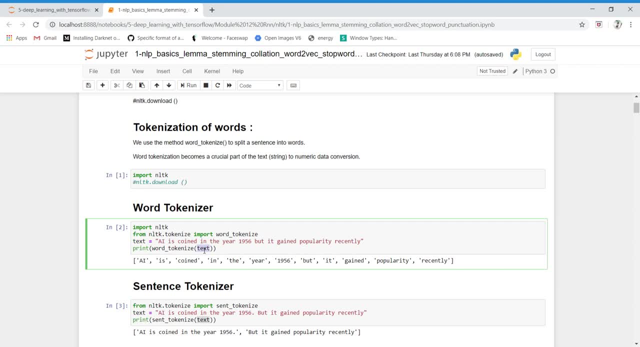 in which you have your sentence which, on which you want to perform this tokenization. So when you check the output of this particular code- so this is the output you'll get- So over here you can see every word is in a single code. That simply means this line get divided into a small, small tokens. So this is. 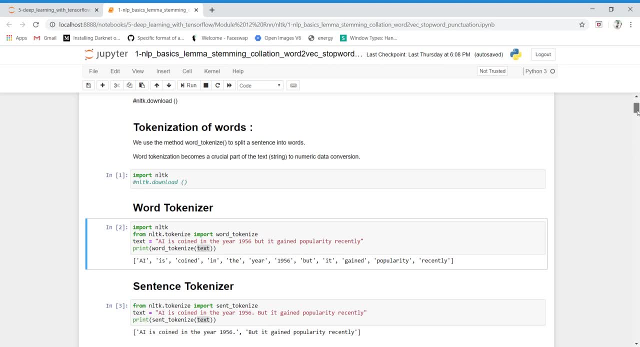 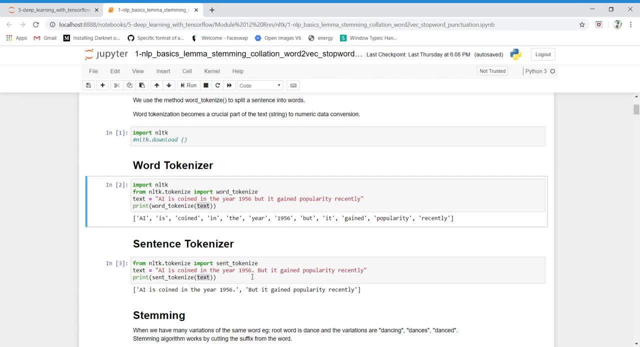 what word tokenization is. Next is sentence tokenizer. Now, what is sentence tokenizer? Sentence tokenizer simply means when you have multiple sentences in a document and you want to separate those sentences. So for that, if you want to perform sentence tokenizer, for that you need. 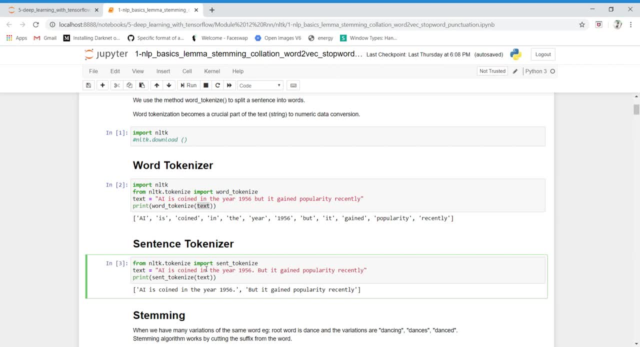 to use this NLTC Tokenize module and from this particular module we are importing this. sent underscore tokenize method right, So text is a variable. In this variable I have two different lines. First line is AI is coined in the year 1956 and the second line is, but it gained popularity recently. So these: 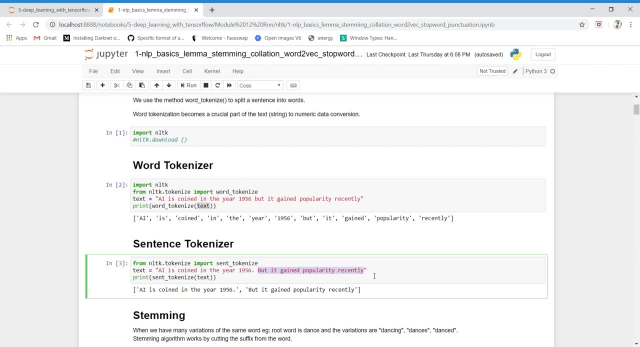 are the two different lines, but it is in a single string right now and we want to divide these two lines. We want to separate these two lines, So this is called sentence tokenizer when we want to separate the lines right. So when you'll apply this sentence: sent underscore, tokenize on the text. 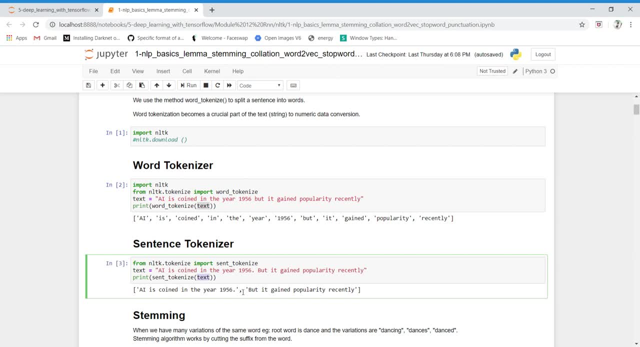 variable which is containing these two lines, you'll get this output. So over here you can see that in single code, first single code, you have one sentence and then second single codes, you have another sentence. So this is what sentence tokenizer does. Now the next. 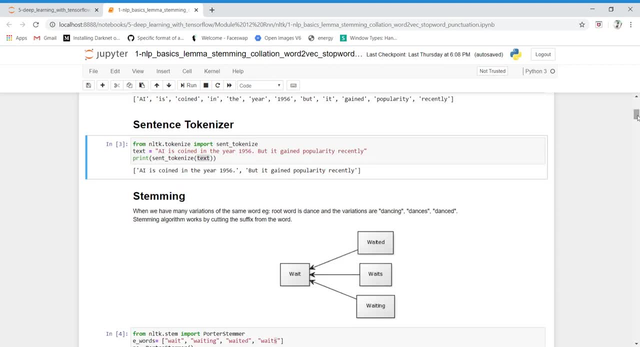 next topic is stemming. Now, what is stemming? So, stemming simply means when you have, you know, you have one root word and you have multiple variants of that word. That simply means a root word is dance, let's suppose, and dancing, dances and danced. These are the three words different. 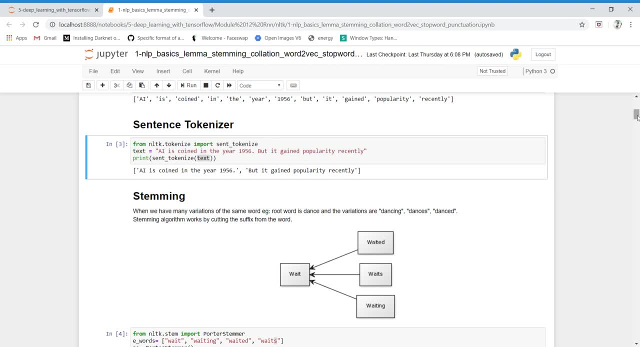 variants of the word dance right. So in NLP we can perform stemming. We always perform stemming when we have multiple variants of single word and we want to convert all those different variants to a single word only. So this is what stemming is and we can perform stemming in natural. 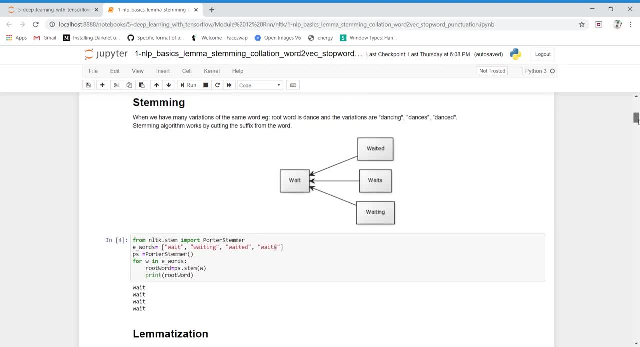 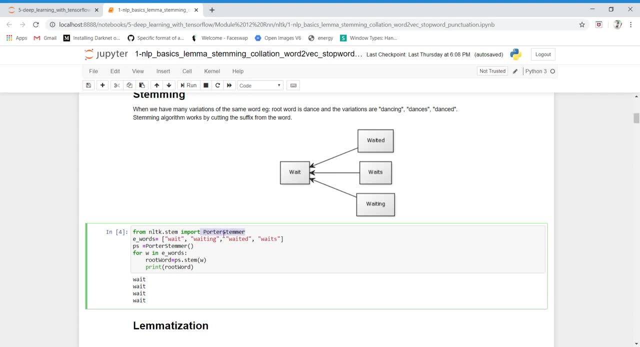 language processing right And the algorithm we can use for stemming is Porter stemmer from NLTK dot stem. I'm importing Porter stem. Porter stemmer is an algorithm with the help of which we can perform stemming, So let's see this. 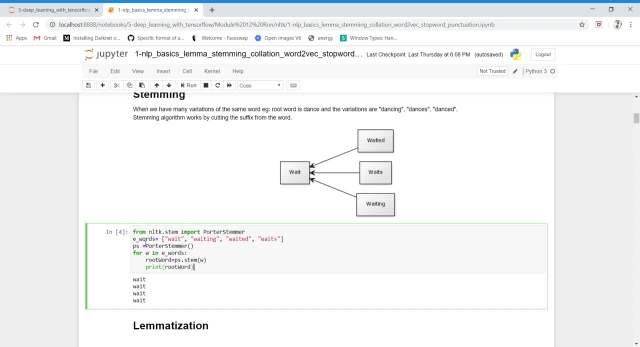 let's see a small example of stemming. So I'm using eWords variable and in this eWord variable I have created one list and this particular list. we have four different values: First is weight, second is weighting and then weighted, and the last one is weights. So 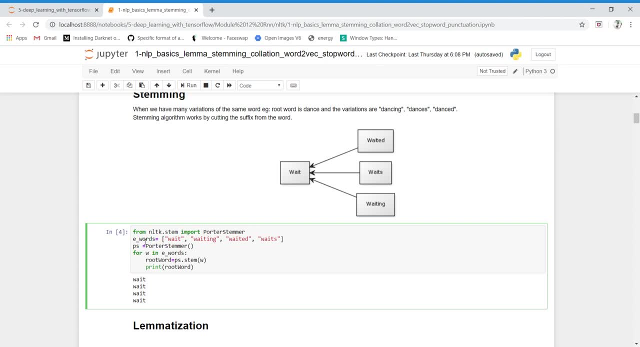 these are the four different values which we have these values in eWords right. So in PS variable I'm calling potter stemmer. That simply means, whenever I want to use this potter stemmer algorithm, I can simply use this PS variable. right Now I'm using a loop. Why? 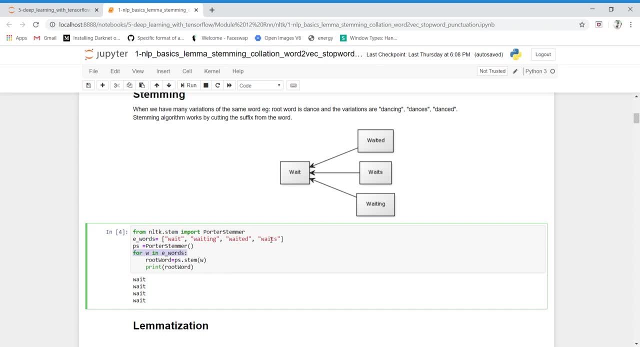 I'm using a loop Because I want to perform stemming on every element of a list, So for that we need to use a loop. So over here I'm again using a different variable with the name of root word, and in this variable I'm using PS. 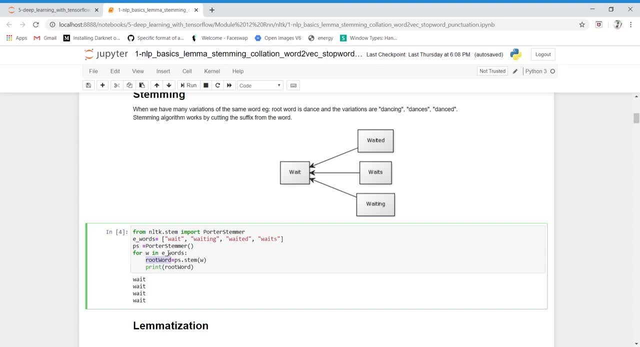 Stem. That simply means PS is potter stemmer Means from potter stemmer algorithm. I'm using stemming method, stem method, and I'm applying that stem method on W, and W is a variable which is responsible to get these values one by one, and then I'm printing the result. So 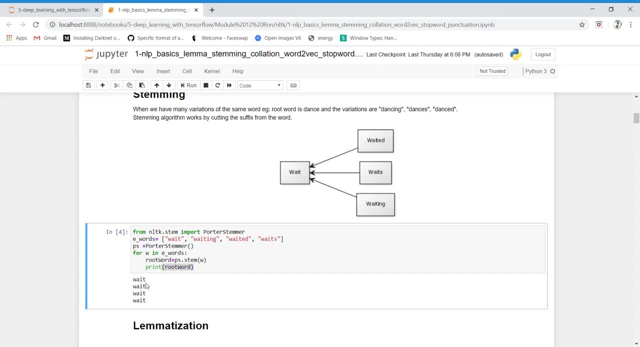 the result of stemming is this. So what happened over here is, instead of this, weighting, weighted and weights. it convert all these three words into a weight. This is what stemming is. Stemming simply means we are cutting down the suffix. So ING is suffix over here, ED is suffix. 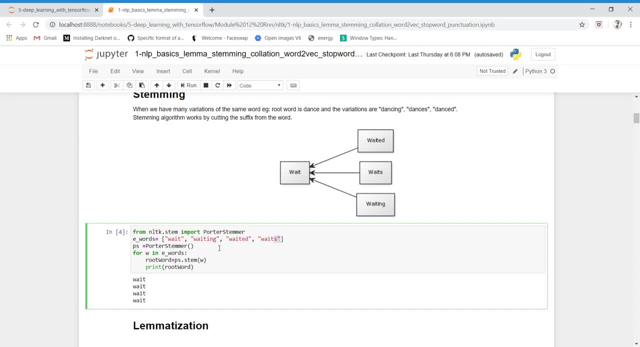 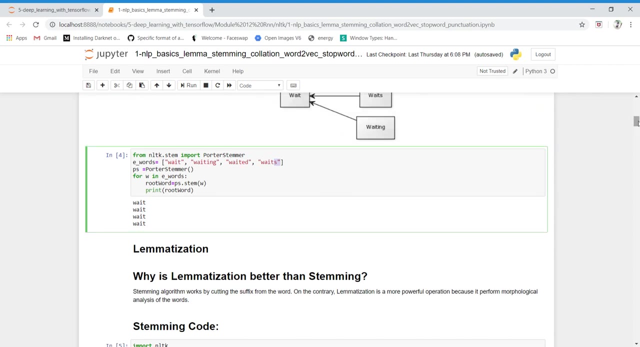 over here and S is suffix over here. So stemming, how stemming converts the multiple variants into a root word by just cutting out the suffixes, right? So this is what stemming. Next topic is lemmatizing. Now, what is lemmatization? So lemmatization simply means it works on the morphological. 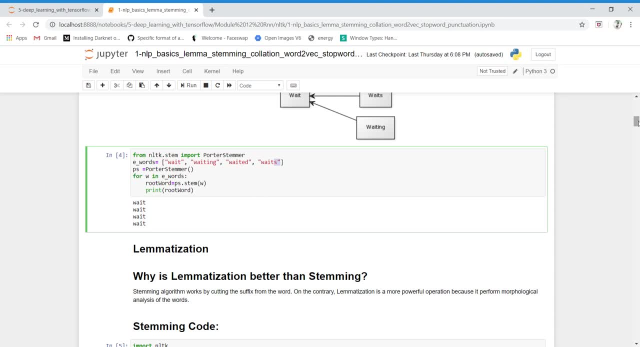 analysis of words, right? So what is morphological analysis? first of all? So morphology simply means when we want to study about words, means how the words are formed, what are the relationship of those words with the other words in the same languages? 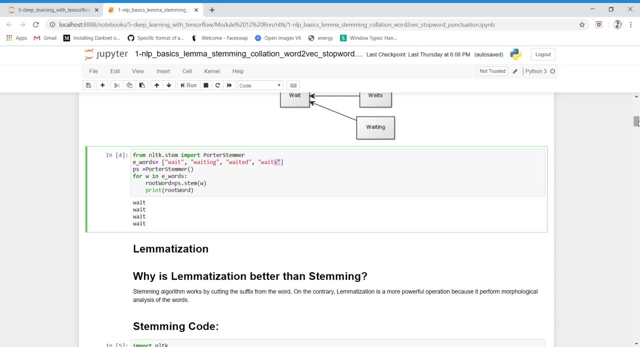 And what are the different prefix values and what are the suffix for that? Basically, morphology simply means analysis of words. study of words means how those words are formed, So these sorts of things comes under morphology, and lemmatization simply means it will perform. 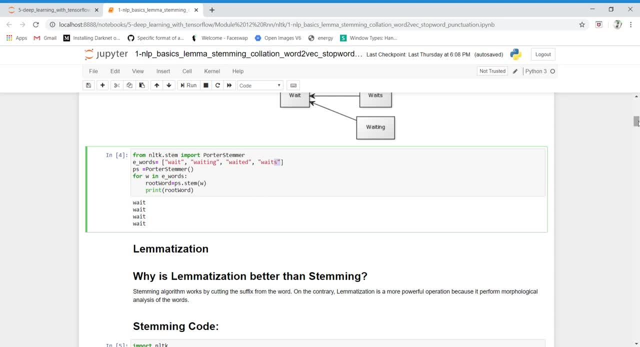 it will convert the multiple variant of words into a single world, but the logic it will use, that will be a morphological analysis- means it will can convert a multiple variant of words into a single word. So lemmatization is simply a form that another kind of homonymous. 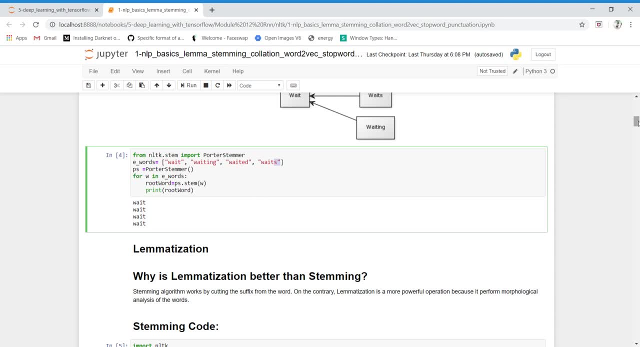 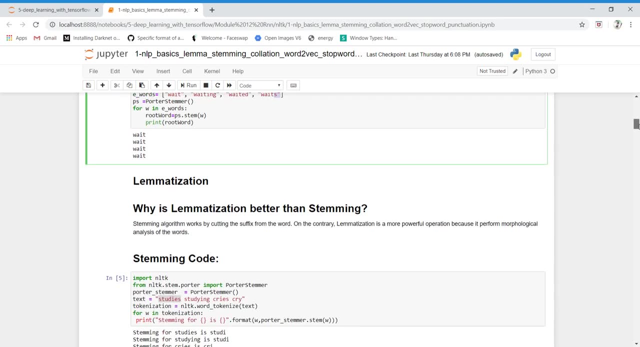 Espero. These are the literally same synonyms, So is more common but also a better analog to have. So lemmatization will understand the words first of all, and after understanding the words it will perform this lemmatization right. So stemming and lemmatization, let's see the difference between. 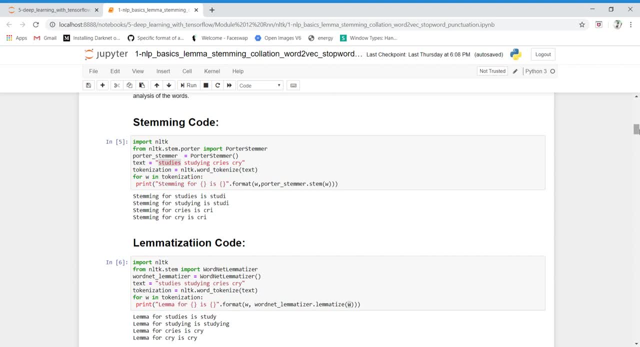 these two Stemming works on the logic of cutting down the suffixes right And lemmatization works on the logic of morphological analysis, means the study of the words right. So let's perform stemming and lemmatization on a single line. So first of all I'm performing stemming, So 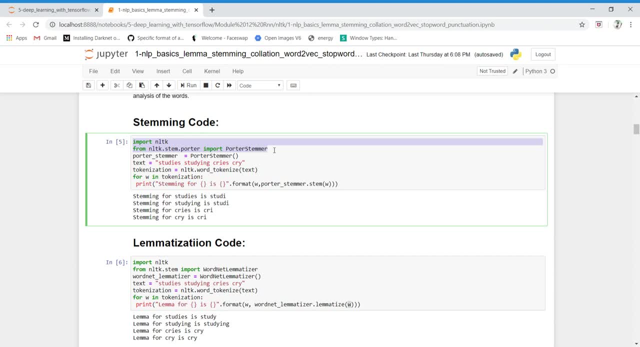 for that again, I have imported all the required modules and I've called this Porter Stemmer algorithm. in this Porter Stemmer variable and text is a variable which contains this line: studies: studying cries and cry On these four words. I want to perform stemming and then I'll 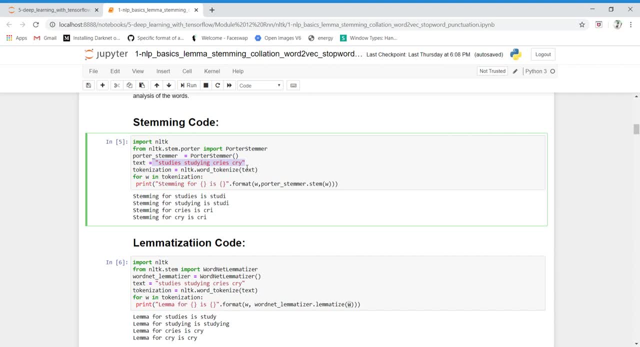 perform lemmatization. So I'm performing stemming and lemmatization on a single line. So if you want to perform stemming or lemmatization, the very first step should be word tokenization. Always remember in natural language processing whenever you want to. 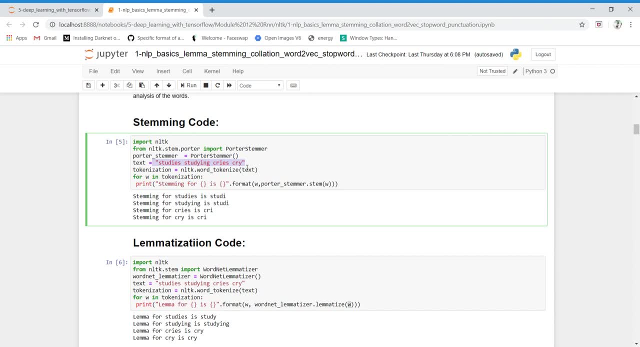 perform any sort of task, you need to divide your sentence into a word first. So that's what we are doing over here. So I'm using word tokenize from NLTK and I'm dividing the sentence into a word. So after performing tokenization, we will perform stemming on it. So over here and we are. 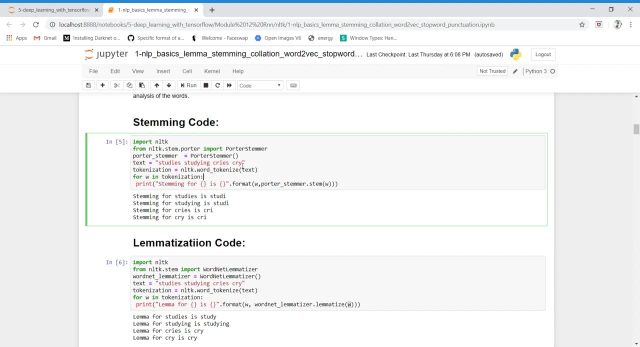 performing in a loop because we have multiple. you know we have four different values on which we want to perform stemming. So that's why we are using a loop, And over here you can see Porter Stemmer dot. stem means I want to use the stem method of Porter Stemmer and I want to use 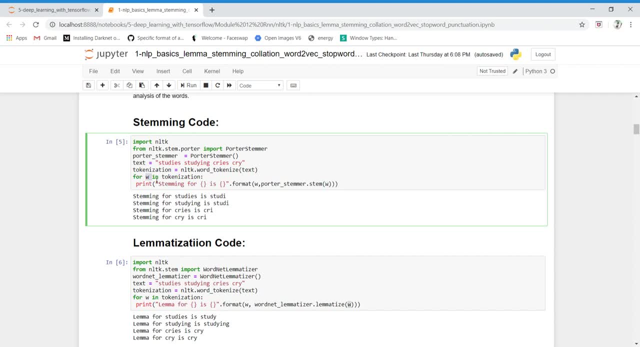 it on W variable. So I'm using the stem method of Porter Stemmer and I want to use it on W variable. And W variable is this variable, and this variable is responsible for getting these four values one by one, And this is the result after stemming Over here you can see like stemming for studies is. 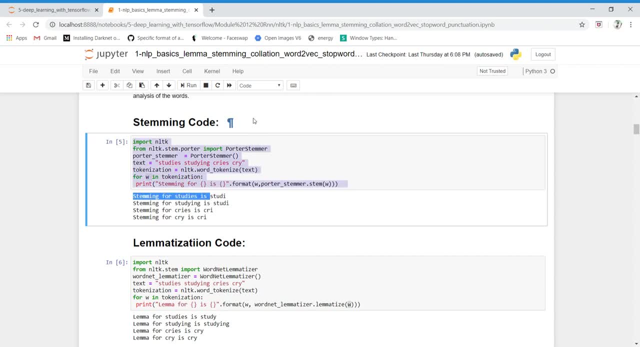 STUDI means this Porter Stemmer algorithm, when performed stemming on studies. So it gives us this output STUDI, And again when it performed stemming on studying, then again it gives us STUDI only. And when it performs stemming on cries. 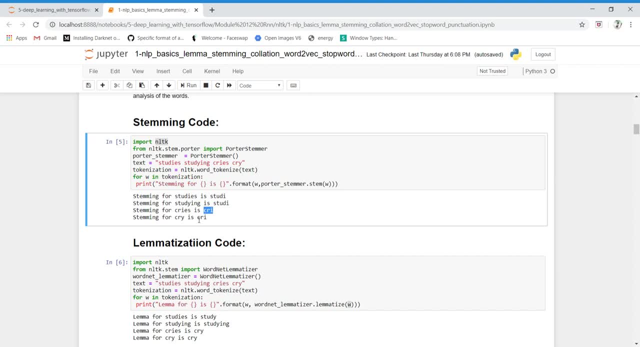 it gives us output as CRI, and for cry also, it gives us CRI. So this is the output which we got when we perform stemming. Now we'll perform lemmatization code on the same line. So we have. 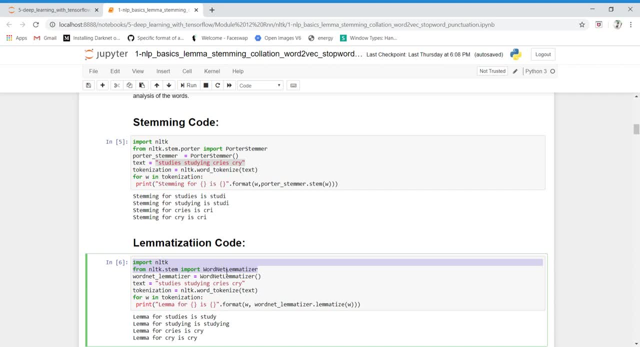 imported the required modules Over here. the lemmatizer we are using is WordNet lemmatizer. WordNet lemmatizer is an algorithm with the help of which we can perform lemmatization. So in WordNet lemmatizer variable I'm calling this WordNet lemmatizer. 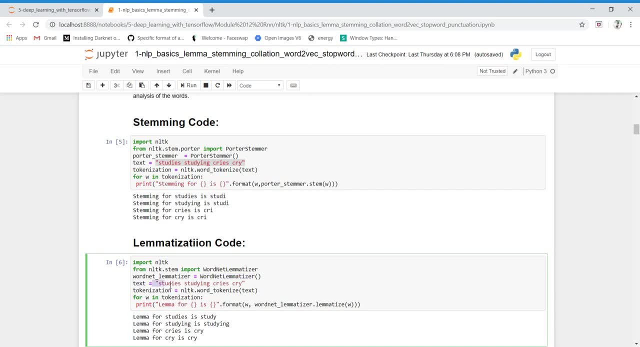 algorithm And text is a variable which is containing this particular line: studies studying cries and cry. This line we have used above, also when we have performed stemming. So again, tokenization is required because, as I've told you like, whenever you want to perform. 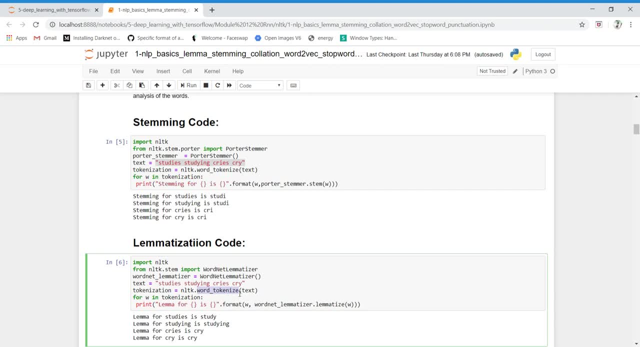 any operation in NLP you need to tokenize the words first- So I have performed tokenization over here- And then WordNet lemmatizer dot lemmatize. That simply means from WordNet lemmatizer algorithm. we want to use this lemmatize method on W variable, which is over here, And 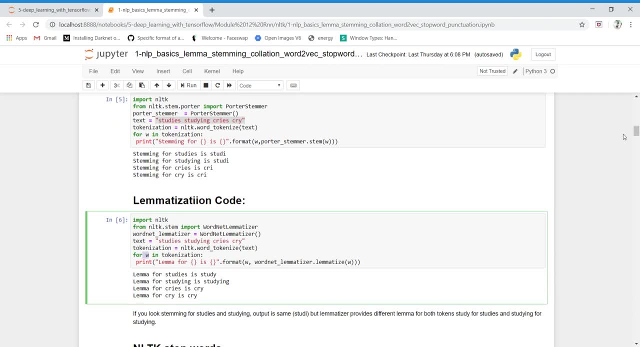 these are the results after lemmatization. So when you'll compare this lemmatization results with the stemming, As a result you'll get to know that lemmatization is giving us more accurate and meaningful output. So that simply means lemmatization is more good as compared to stemming right. 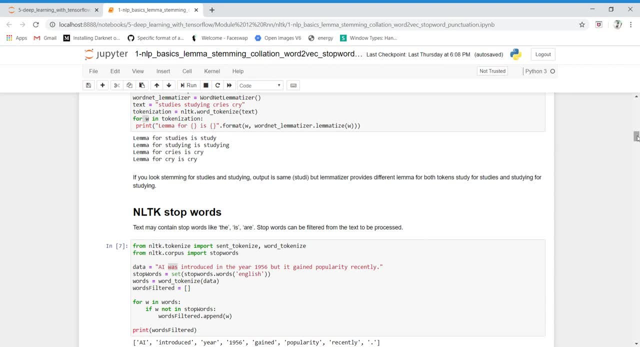 So the next topic is stop words. Now, what are stop words? So stop words are the words which which are used very commonly in every document like this: is, are, are, but in the right, These are the stop words. So in our documents, in our text, in our sentences. 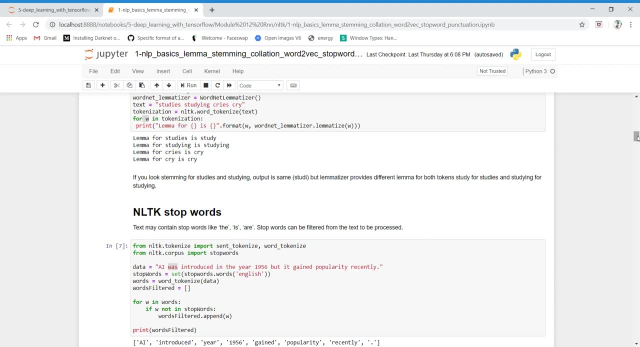 there are lots of stop words which are not actually useful when you want to perform some- you know- predictions or analysis. So we want to delete stop words. So for that we have a separate module with the name of stop words. So this module is responsible for. 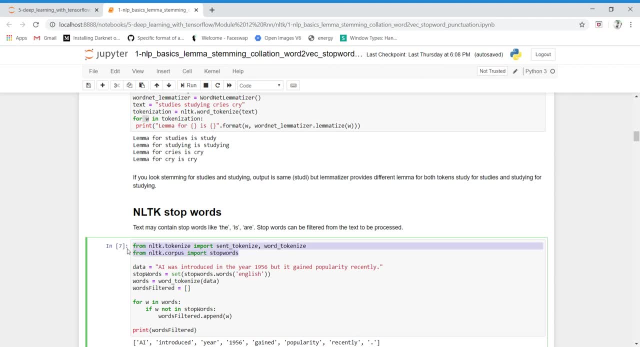 removing all the stop words. So I have imported all the required stop words. So I have imported all the required modules. and data is a variable in which I have a sentence on which I want to perform a stop word operation and then I have another variable with the name of stop words and this: 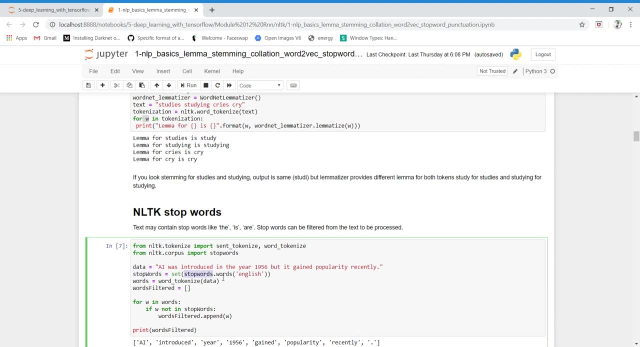 in this variable. I'm calling stop words dot words. Stop words is a module name. Dot words is a method of it means from stop words I want to use words. Which word I want to use? Which belongs to English dictionary? 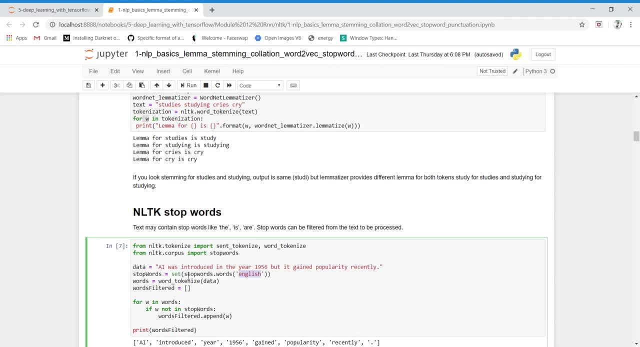 And I want to store those stop words which belongs to English dictionary in a stop word variable right Now in words. So again, this is a line. So if you want to perform stop words operation also, then again you need to tokenize the line first of all. right, 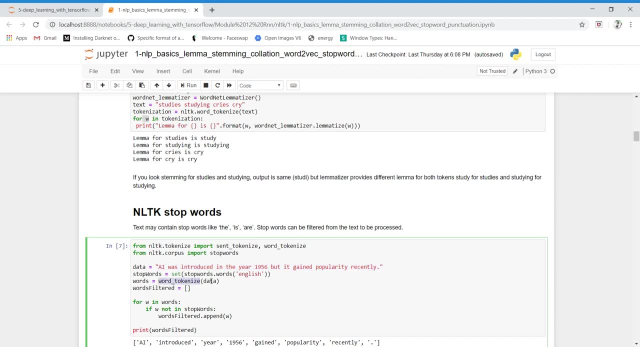 So that's why we are using word tokenize over here on a data variable, data variable which is containing a line. So after word tokenization, all the separate modules, all the separate modules, all the separate words got stored in words variable. Now we have a blank list. This in this list: 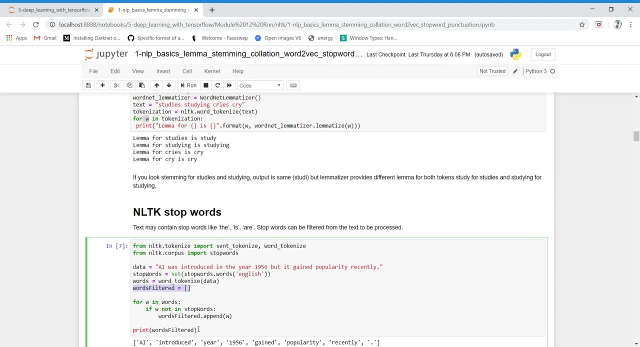 we will be storing the results after the whole program. Now I'm using a loop. Why I'm using a loop? Because we have multiple different words and we want to work on every word, and that's why we are using a loop. In this loop, I'm using a condition, and the condition is if that word not in stop words. 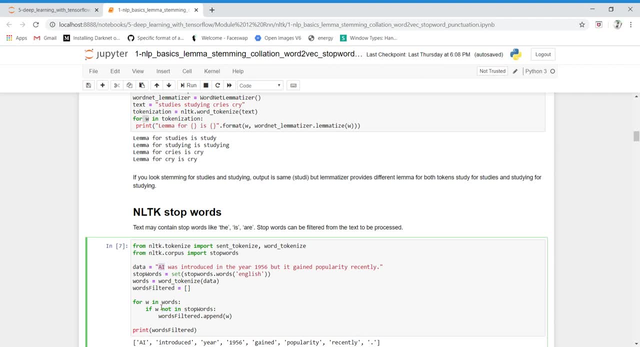 that simply means the very first word is AI. If AI not in stop words, then in this word filtered list- we want to append that list and we want to store that word in this particular list Means AI will get stored in it, because AI is not a stop word. 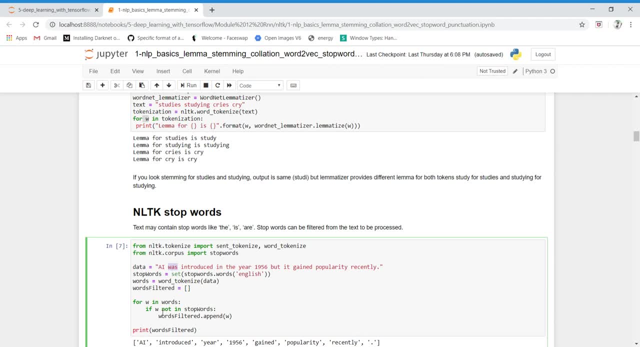 And then the second word is was. So if was not in stop word, then that word should get stored in the list, and if word this was is a part of stop words, then it will get eradicated. so this is how, for every single word will perform the functionality, and this is the final result which 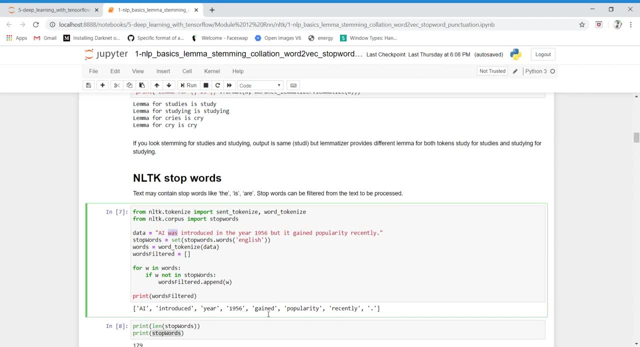 will get ai introduced. year 1956 gained popularity recently, so we'll see the result and if we'll match this result with the current exact line- actual line, so you'll see- was in the but and it is missing from the output. why these words are missing from the output? because these words are: 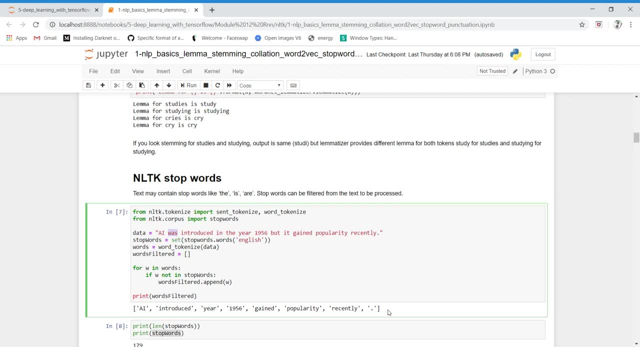 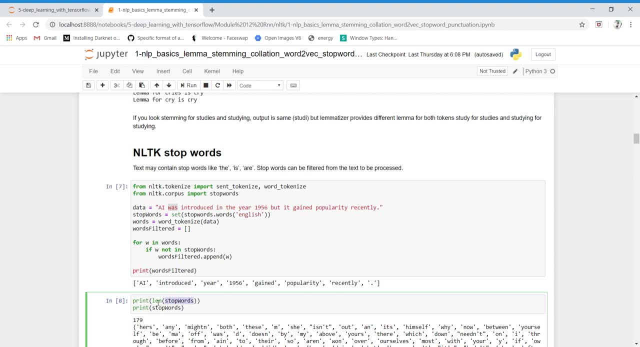 the stop words. so this is how we can use stop words. so let's suppose, if you want to see the means, how many, uh, different stop words are there? so you can simply use alien length method and then the stop word variation name in which we are storing stop words of English. so this will give you the